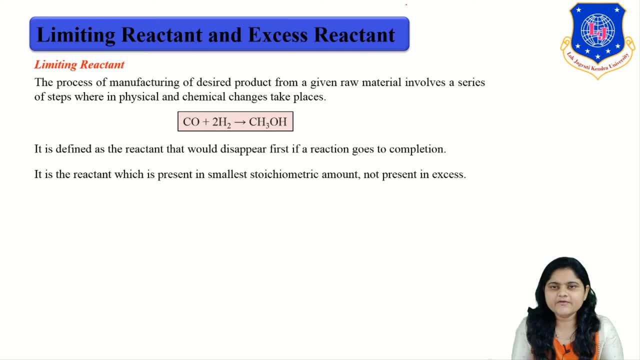 reaction between CO plus H2 will give us CH3OH. Now let us assume 100 kilomole of CO and 200 kilomole of H2 is initially taken, So as reaction goes towards the completion, CO and H2 would. 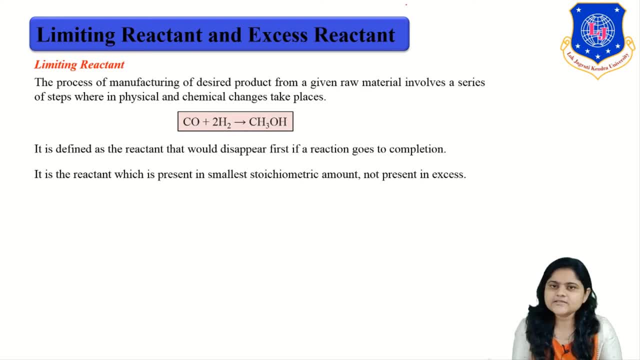 disappear at the same time. But instead of that, let us assume 100 kilomole of CO and less than 200 kilomole of H2 in our system. So what if reaction goes towards the completion? H2 will disappear first, because we are feeding H2 in a less stoichiometric amount as compared. 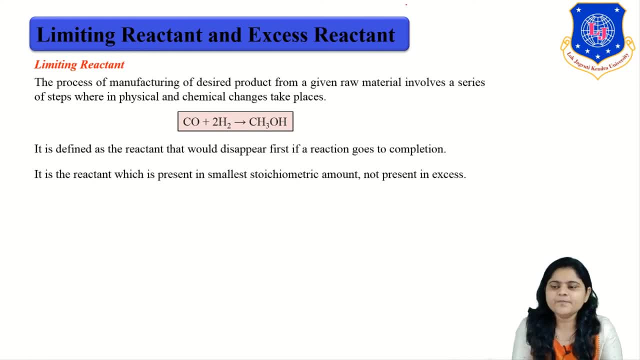 to its requirement. So in this case, H2 will be our limiting reactant. Works of that if we are applying a less amount of CO is compared to their stoichiometric amount, and enoughических amount of CO would be the limit reaction. If this happens, in return, that will十 percent. before. I am applying a less beaucoup amount of CO as compared to this stoichiometric amount, and myself do not. I can get such a solution, that is, it becomes accurate after I try to be able. torels: the H2 is an essential component. Step 3. Ensure thatот or take care all the left. 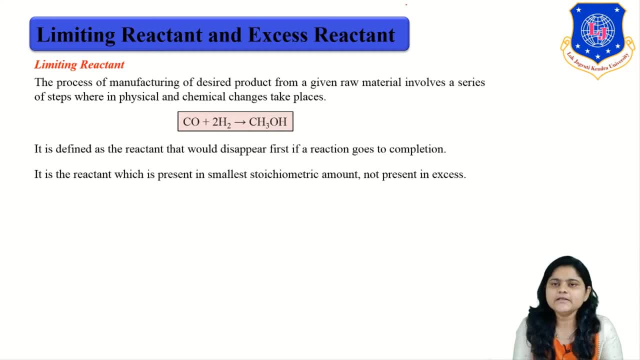 of H2.. So CO will be the limiting reactant in that case. So in brief, I can say that limiting reactant that means the reactant that would disappear fast if reaction goes towards the completion, The reactant which is present in the smallest stoichiometric amount, which is not 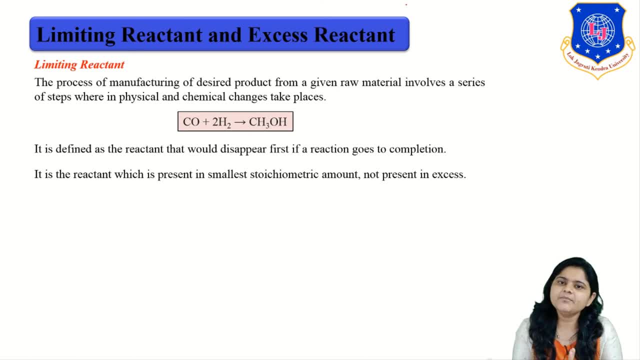 present in the excess. that is known as the limiting reactant. Now let us say the excess reactant. Excess reactant, that means reactant which is present in the excess of its theoretical requirement, or I can say the reactant which is present in the more amount as compared to its. 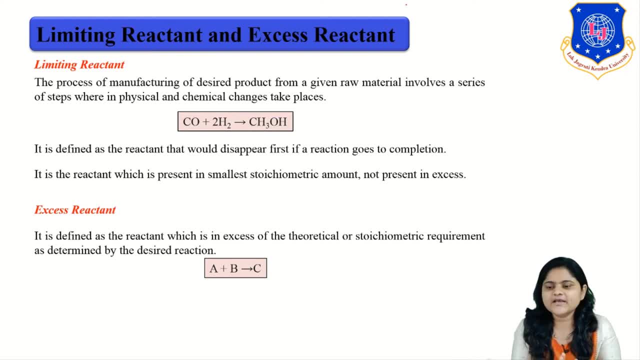 the stoichiometric requirement, So which is known as the excess reactant. Say, for example: A plus B gives C, So percentage excess B is equal to moles of B supplied in feed, minus theoretical requirement of B divided by moles of B. So this is called the limiting reactant. So 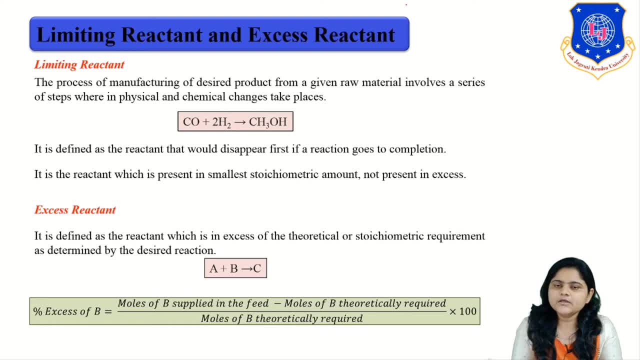 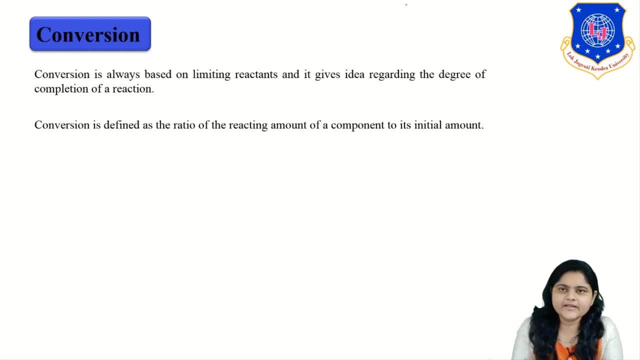 moles of B theoretically required, multiply it with the 100.. Now see the conversion. Conversion is always based on the limiting reactant and the conversion gives the idea about the degree of completion of any chemical reaction. So whenever we are calculating the conversion, 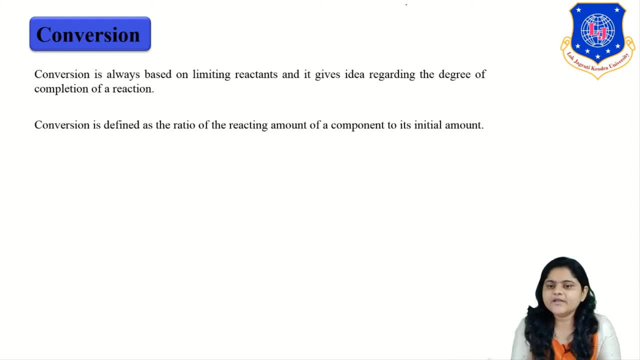 conversion will always be based on the concentration of limiting reactant. So conversion that means ratio of reacting amount of any component to its initial amount taken. So how we can calculate the conversion? Say, for example, reaction A plus B gives C. So percentage conversion of A is equal to. 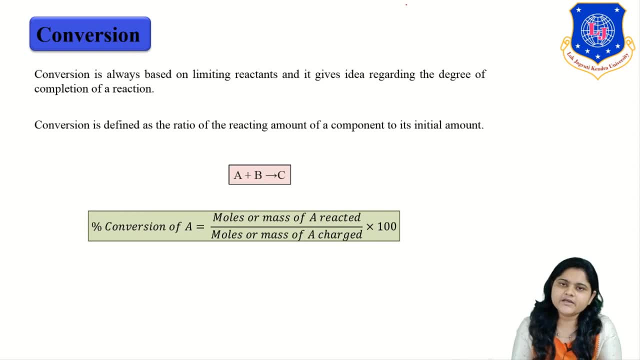 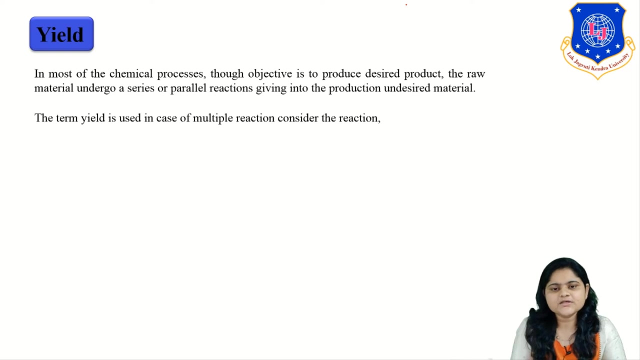 moles over mass of A reacted divided by moles over mass of A initially charged in the system, multiplied with the 100. So by this way we can calculate the percentage conversion of a reaction of patients in the extremity. So this is the 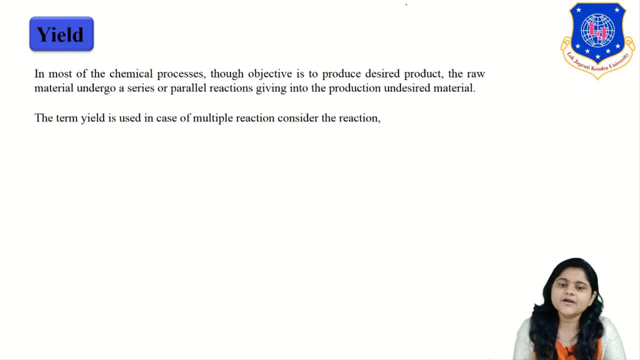 contribution of R materials to the CPT and to theissa fluoride, Следed By l Chinese Chinese. this: if a reaction is A plus B gives C and B plus C gives D, where C is our desired product and D is our undesired product and component A is our limiting reactant. So percentage: 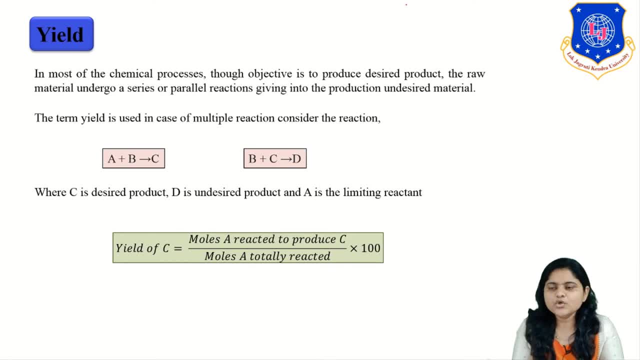 yield of component C is equal to moles of A reacted to produce C. C is our desired product divided by moles of A totally reacted, multiplied with the 100.. So percentage yield of any substance is always calculated based on the desired product and the undesired product. Next terminology: 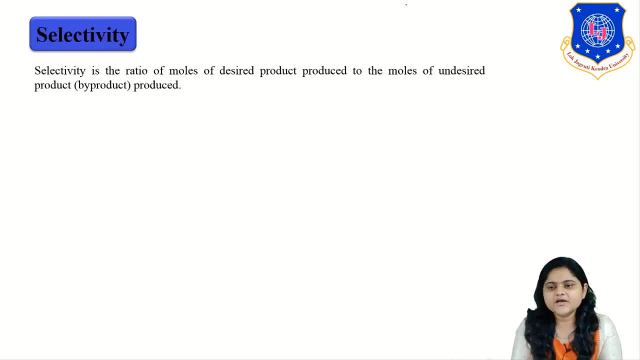 is the selectivity. Selectivity means a ratio of moles of desired product produced to the moles of undesired product produced. In the other terminology I can say the ratio of the moles of undesired product produced to the moles of undesired. 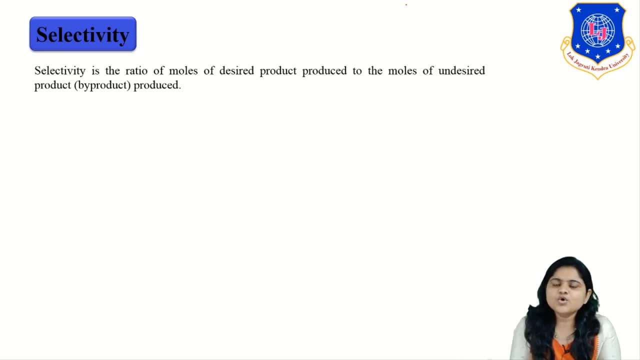 can say that selectivity is a ratio of moles of limiting reactant reacted to produce desired product divided by moles of limiting reactant reacted to produce undesired product. Say, for example, a reaction A gives C and A gives D, where C is the desired product and D is the undesired. 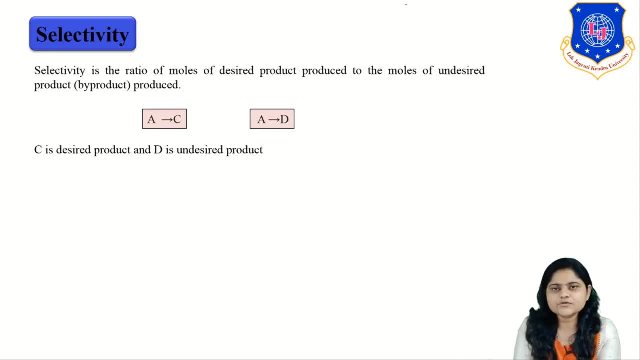 product. So selectivity is a ratio of moles of desired product to the moles of undesired product. that means selectivity of C relative to D is equal to moles of C formed divided by moles of D formed. If yield of any chemical reaction is 100 percent, that means we can say selectivity of that. 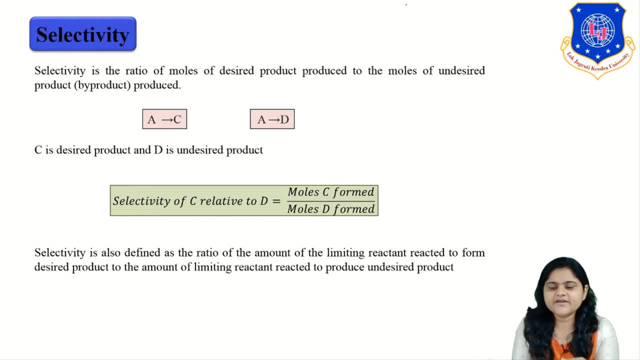 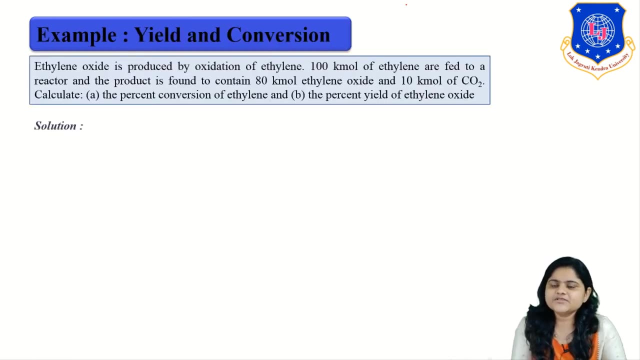 reaction is 1.. We can say that selectivity is also a ratio of limiting reactant Reacted to produce desired product divided by limiting reactant reacted to produce undesired product. So this was the basic terminologies to calculate any material balance problem which. 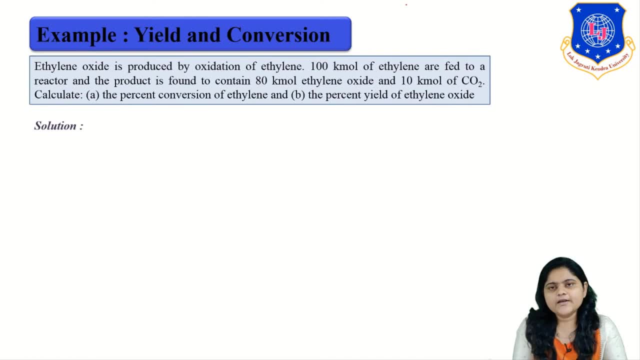 involves chemical changes. Now we will solve example phase of that. Ethylene oxide is produced by oxidation of ethylene. Hundred kilo moles of ethylene are fed to a reactor and the product is being produced. This reaction is called the reaction, reaction of the reaction. 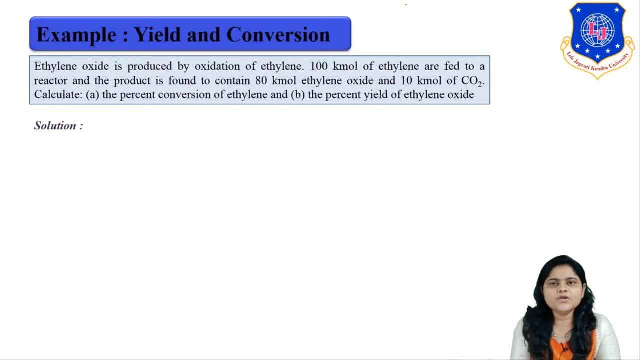 C and A of the reaction. reaction are treated to a chemical reaction, So the reactant is product is found to contain 80 kilomole ethylene oxide and 10 kilomole carbon dioxide. Calculate number 1, the percentage conversion of ethylene and number 2, the percentage yield of ethylene. oxide. Ethylene oxide is produced by the oxidation of ethylene. 100 kilomole of ethylene is initially taken and product is 80 kilomole ethylene oxide and 10 kilomole carbon dioxide. This thing is given to us. Now we need to calculate percentage conversion of ethylene. What is the formula for? 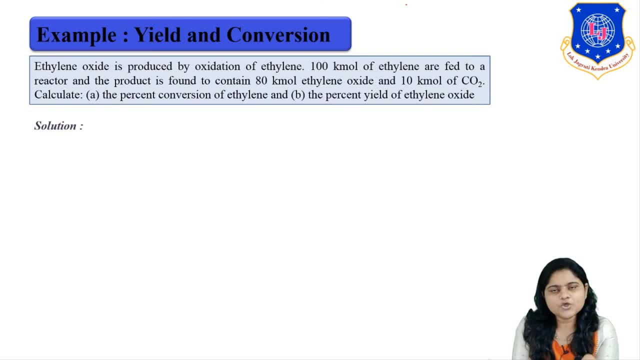 that Percentage conversion of ethylene is equal to moles of ethylene reacted divided by moles of ethylene charged multiplied with the 100.. Now to calculate percentage conversion: moles of ethylene are equal to moles of ethylene charged multiplied with the 100. 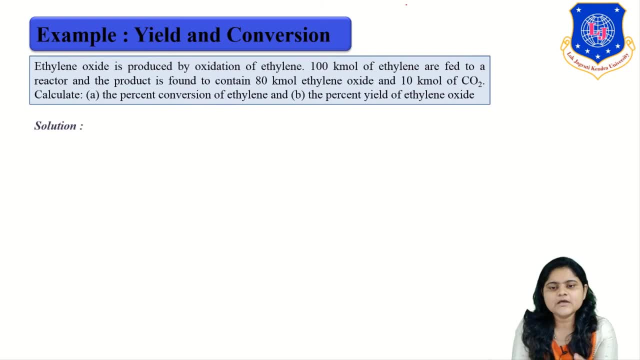 So moles of ethylene charged are required, but it is given which is 100 kilomole. Now we need to calculate moles of ethylene reacted, One reaction in which ethylene is oxidized to produce ethylene oxide. Any other reaction, ethylene plus oxygen- will give us carbon dioxide. 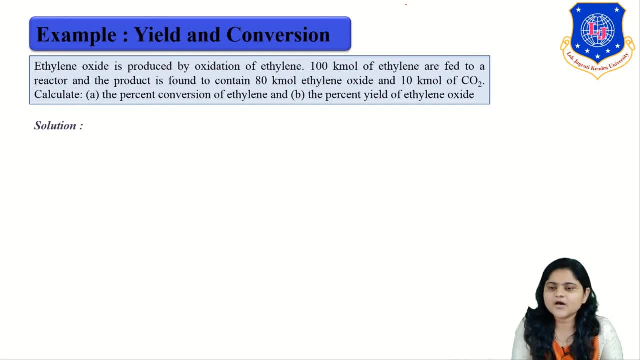 So let us write these two calculations and find the amount of ethylene reacted. Let us say reaction number one, which produce ethylene oxide. So ethylene plus 1 by 2 O2 will produce ethylene oxide. Here amount of ethylene oxide that get produced is 80 kilomole. So according to this, 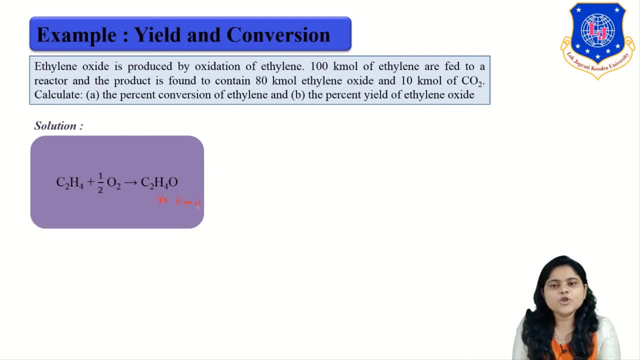 documentary amount, I can say that 1 kilomole ethylene oxide is get produced from 1 kilomole ethylene, So 80 kilomole ethylene oxide is produced from 80 kilomole ethylene oxide. So 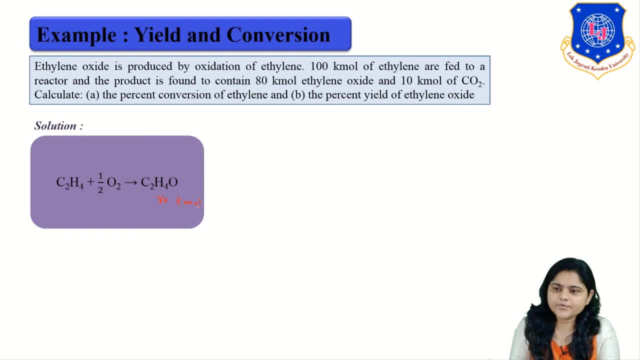 ethylene reacted to produce ethylene oxide is equal to 80 kilomole. This is for the reaction number one. Now reaction number two, which produce carbon dioxide. So ethylene plus oxygen will give us carbon dioxide plus H2O. Now where is the chemical reaction From this chemical? 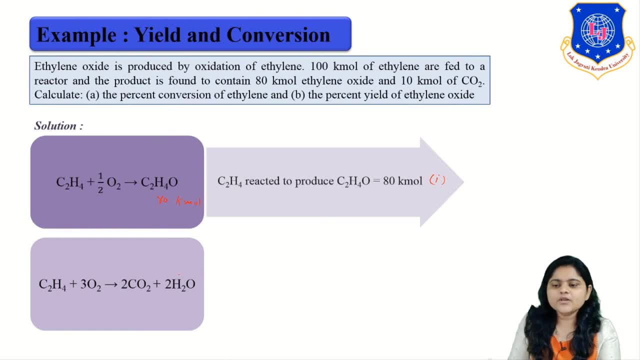 reaction, I can say that 2 kilomole ethylene oxide is equal to 80 kilomole ethylene oxide, So we can say that 2 kilomole carbon dioxide is getting produced from 1 kilomole ethylene. 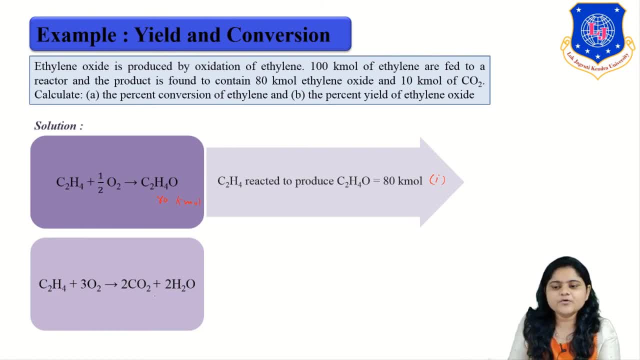 Here the amount is 10 kilomole carbon dioxide is get produced. So I can write a equation like this: 2 kilomole carbon dioxide is produced from 1 kilomole ethylene, Therefore 10 kilomole. 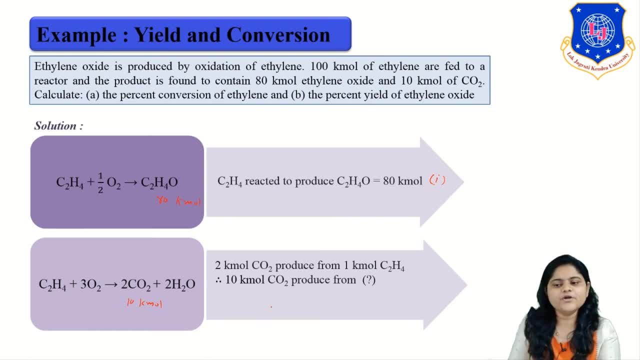 carbon dioxide produced from what amount of ethylene? So ethylene reacted to produce carbon dioxide is equal to 80 kilomole H2O. So the reaction number one, which produce ethylene equal to 10 divided by 2, that is 5 kilo mole. This is for reaction number 2.. Now ethylene. 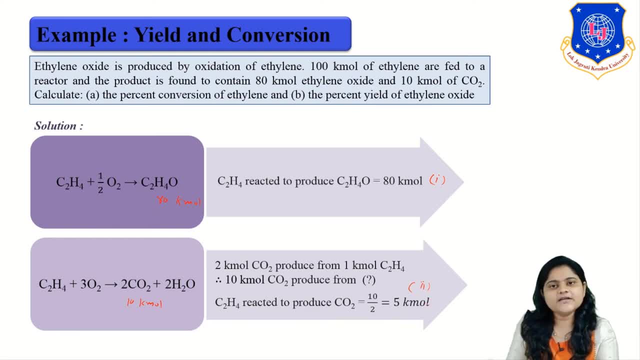 oxide is our desired product and carbon dioxide is our undesired product. So ethylene is reacted in both the product, desired product, as well as undesired product. So total ethylene reacted is equal to 80 plus 5, that is 85 kilo mole. So how we can calculate concentration. 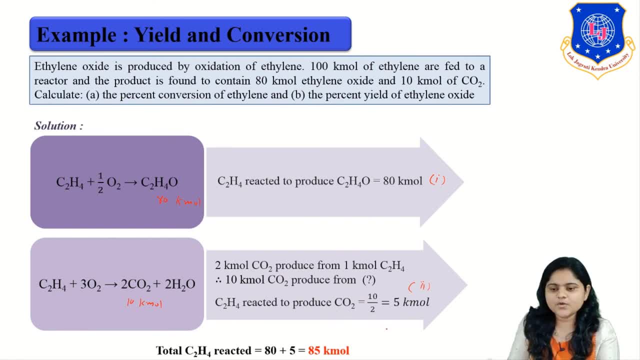 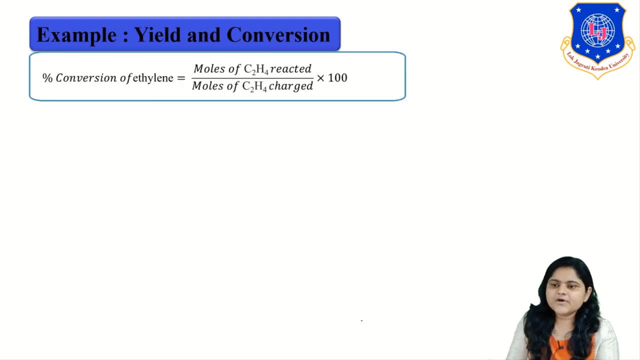